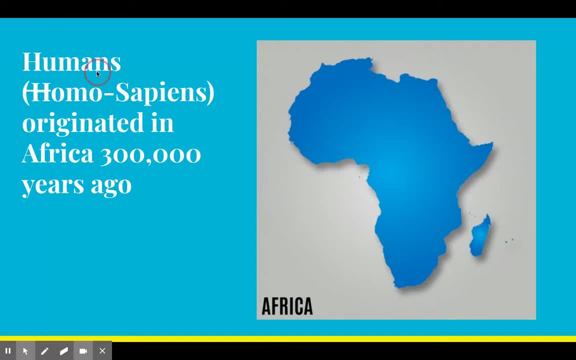 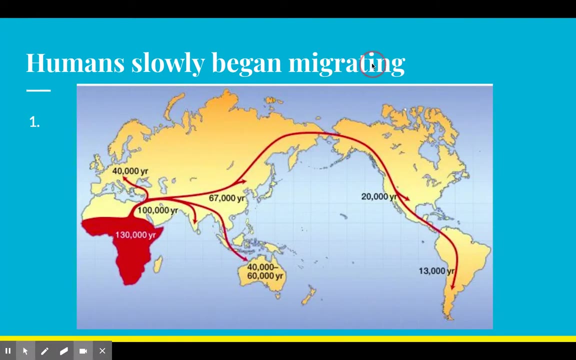 So humans- evidence of humans was first found in Africa. So it started. it began originated in Africa 300,000 years ago And then humans slowly began migrating. So this is a map and we follow the red arrows as to where humans migrated. So, like we just said, humans started in Africa. 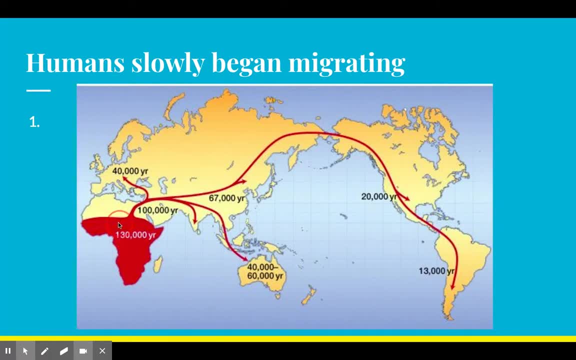 That's where they originated. And then we follow the red arrows as to where humans migrated. That's where they originated And then, 100,000 years ago, they moved out of Africa and started to come into Asia, And they moved 67,000 years ago up into Asia. They moved 400,000 years ago up. 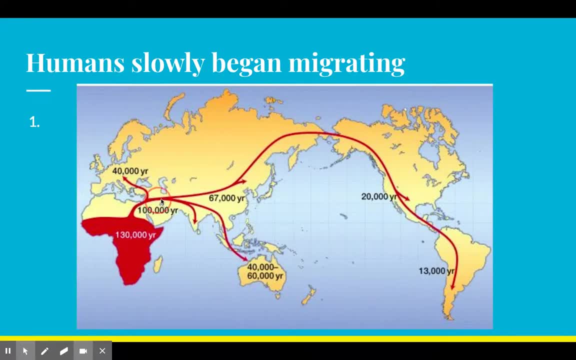 into Europe. They also moved south, down into more parts of Asia, into Australia, And as the time kept passing they moved up north, crossed the land bridge, 20,000 years ago in North America and 13,000 years ago in South America. But all humans, there is evidence that they started in. 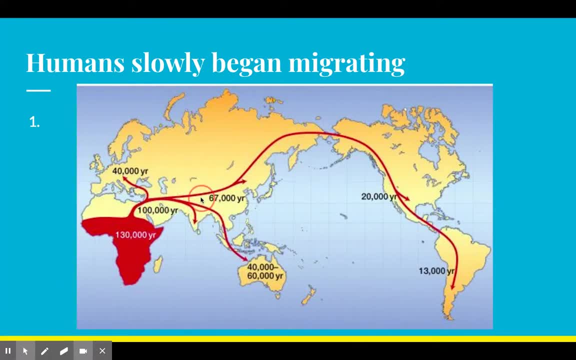 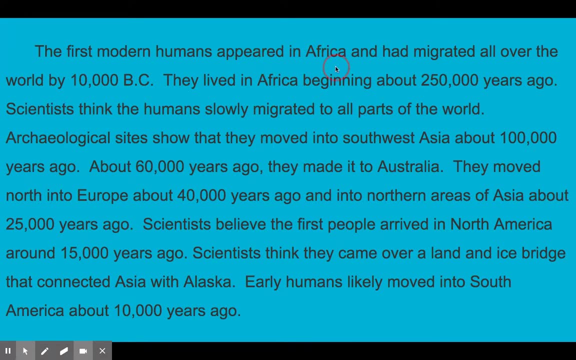 Africa first, before moving to all the other continents. The first modern humans appeared in Africa And had migrated all over the world by 10,000 BC. They lived in Africa beginning about 250,000 years ago. Scientists think the humans slowly migrated to all parts of the world. Archaeological sites: 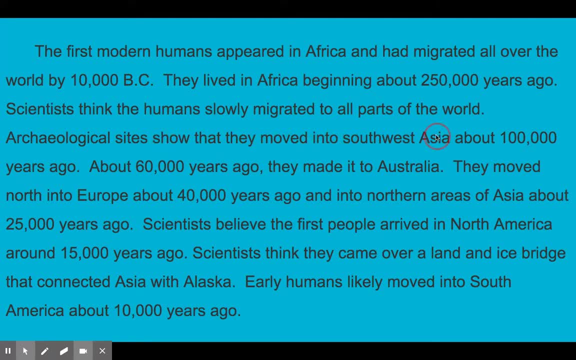 show that they moved into Southwest Asia about 100,000 years ago. About 60,000 years ago they made it to Australia. They moved north into Europe around 40,000 years ago and into northern areas of Asia about 25,000 years ago. Scientists believe the first people arrived in North. 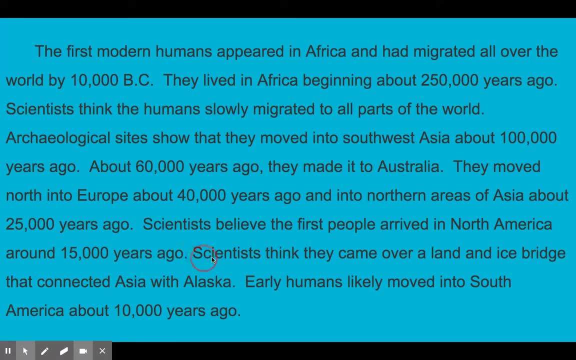 America around 15,000 years ago. Scientists think they came over a land and ice bridge that connected Asia with Alaska. Early humans likely moved into South America, Australia and California. The only new überzeuging evidence was that scientists came over the ice bridge that connected Asia.